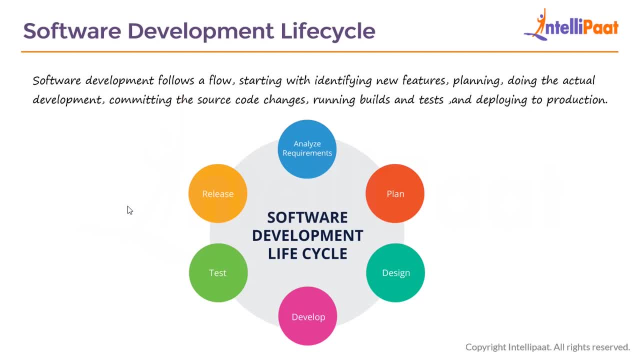 the agile software development model was introduced. Agile changed the way software development teams work. One of the key principles of this methodology was delivering working software frequently. The focus moved to releasing incremental software rather than the Big Bang waterfall releases, which took months and even years. 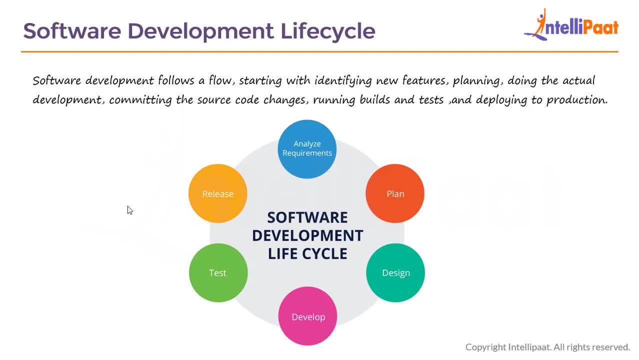 So delivering software frequently meant producing stable code for every incremental release. It was quite a challenge to integrate changes from various developers on the team. This led to software teams looking for better approaches, Continuous Integration, or CI. it offered a ray of hope and started to gain in popularity. 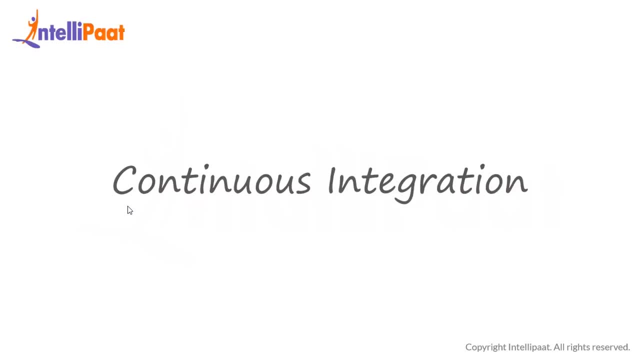 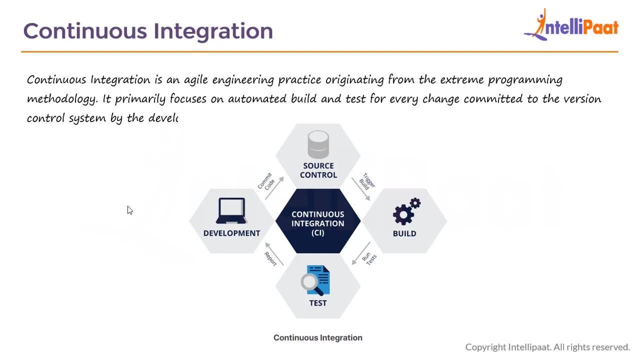 Now let us see what continuous integration exactly is. There is more to the next topic. So continuous integration is an agile engineering practice from the extreme programming methodology. It primarily focuses on automated build and test for every change committed to the version control system by the developers. 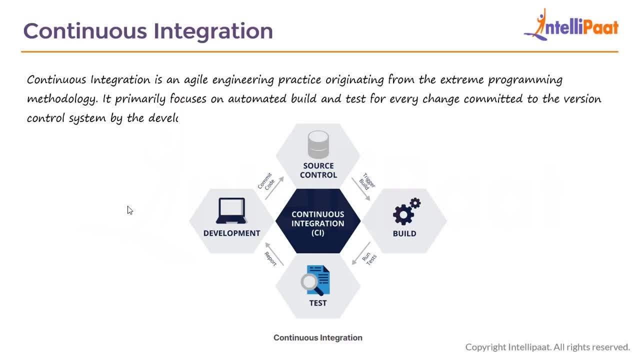 And, according to Martin Fowler, continuous integration is a software development practice where members of a team integrate their work frequently. Usually, each person integrates it At least once a year, Leading to multiple integrations per day. Each integration is verified by an automated build. 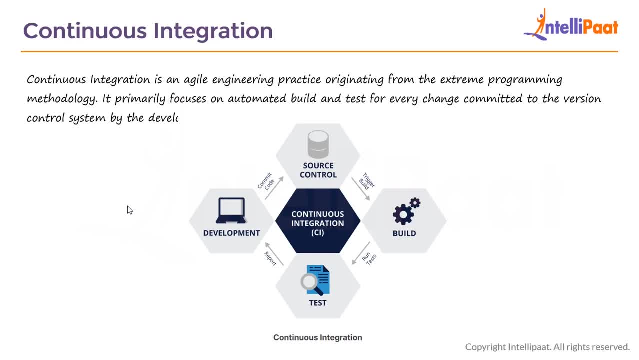 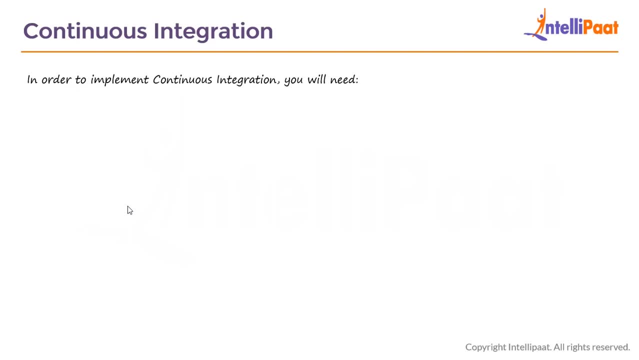 This includes the testing process as well- And then to detect integration errors as quickly as possible. In order to implement continuous integration, you will need the following: Firstly, you will need a version control system, So VCS. it stores all the source code checked in by the teams and acts as a single source. 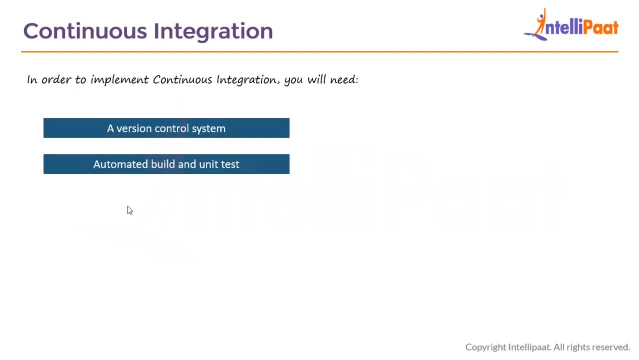 of truth. Later you will need automated build and unit test. It is not sufficient if the code written by a developer works only on his or her machine. Every commit that makes it to the version control system should be built and tested by an independent continuous integration server. 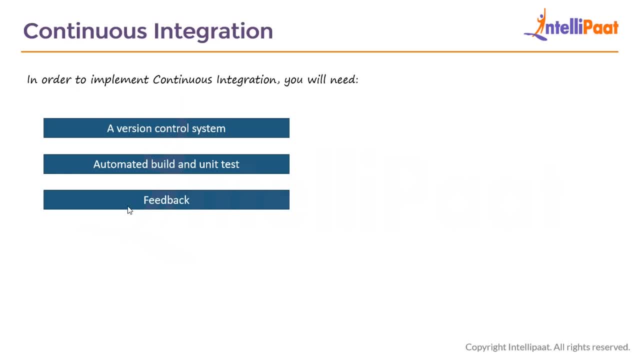 Then you will need some form of feedback, So developers should get their feedback on their commits. Anytime a developer's change breaks the build, they can take the necessary action, for example, email links etc. And finally, you would need an agreement on the base of working. 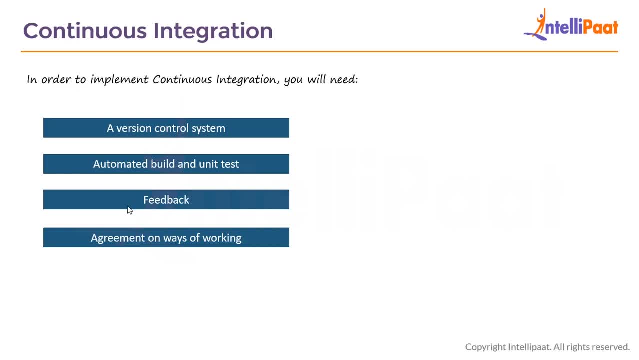 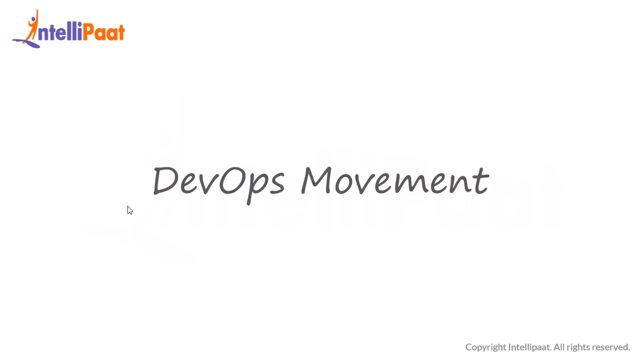 It is important that everyone on the team follows the practice of checking in incremental changes, rather than waiting till they are fully developed. Their priority should be to fix any build issues that may arise with the checked-in code. Now that we have an idea about continuous integration, let us move on to the next topic. 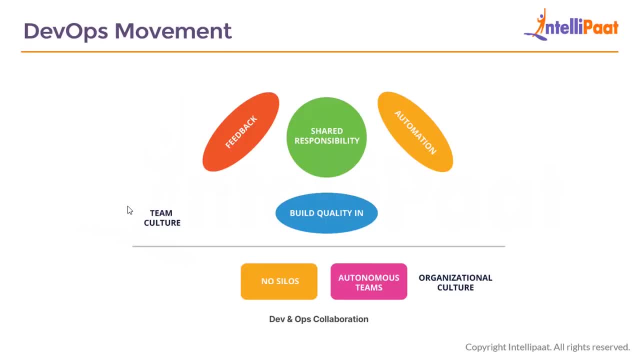 which is the DevOps movement within CI CD. So Continuous integration primarily solves the development part of the workflow. However, there is more to the software delivery than just feature development and integrating the changes. There is testing, which involves manual testing and automated testing as well. 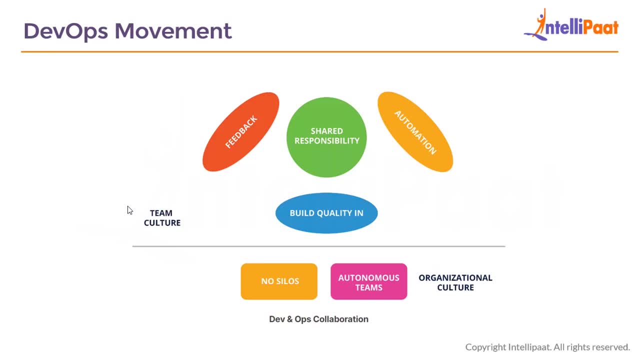 And then release process, where the actual deployment to the customer or production takes place. And in the previous DevOps era, each team was responsible for their own work. The development team would take care of the feature development. This is where their job ended. 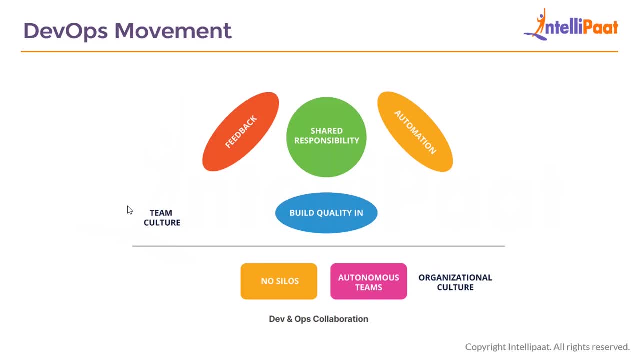 They would then throw it over to the quality assurance or the QA team. The QA team would run all the extended test suites which can be manual and automated, And then, if things worked out fine, they would hand the features off to the operations team. 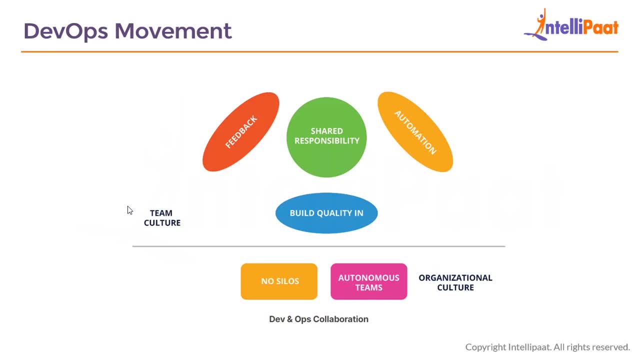 who would then ultimately roll out the new features into production and manage them. Each of these teams worked in silos, which means independently. The release processes were mostly manual And error-prone, leading to longer and painful release cycles. Every time something went wrong, a massive amount of time was spent trying to get rid. 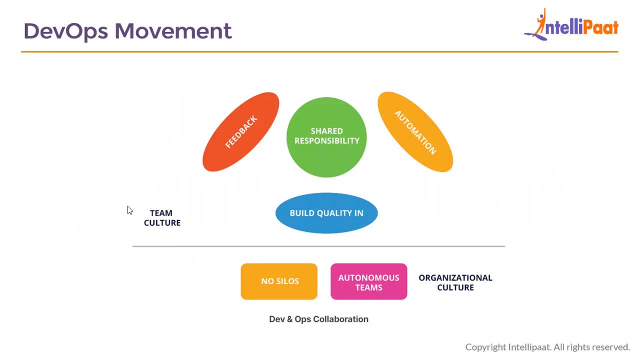 of the root cause of the issue, let alone the blame game. All this resulted in a lot of wasted time at various levels of the organization. In reality, every single team should be equally responsible for the release of the new software, which means that all of these teams need to work in close collaboration with each other. 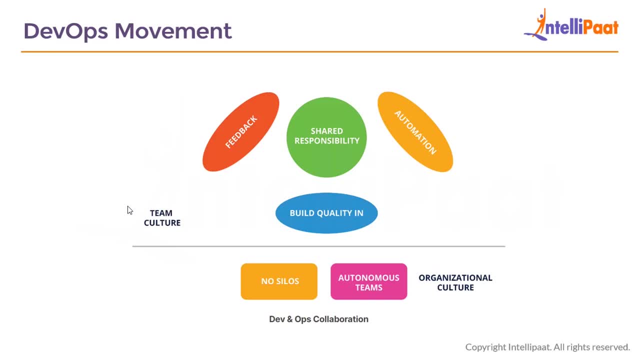 The DevOps movement, which also includes the development of the new software, is a big part of the development process. The development process, which originated from agile software development, strongly emphasizes the need for collaboration amongst the various teams involved in the software delivery process. 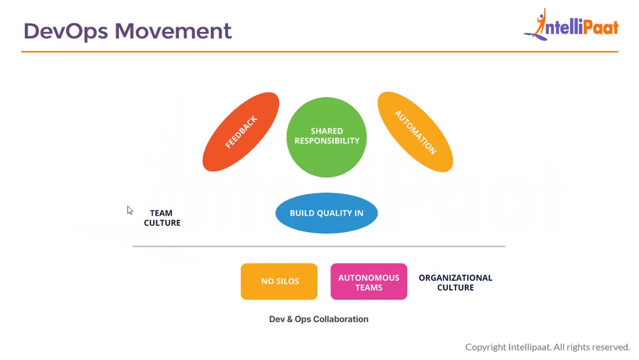 In addition to close collaboration, automation of each of the stages of the software delivery process and constant feedback cycles are also considered extremely important. Continuous delivery provides a framework to achieve the goals of DevOps through automation and continuous feedback loops. So this is it. 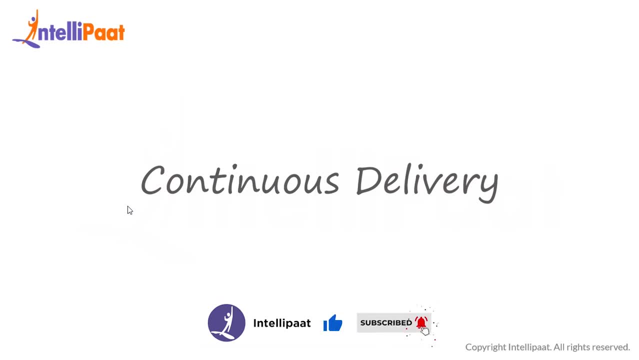 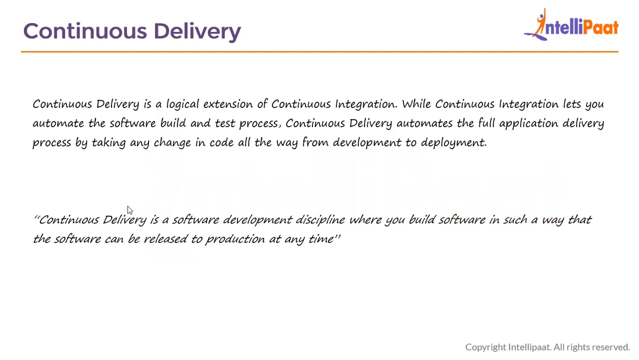 This is what the DevOps movement held, and let us move on to the next topic, which is continuous delivery, or the CD part of the CI-CD pipeline. Continuous delivery is a logical extension of continuous integration. While continuous integration lets you automate the software, build and test processes, continuous 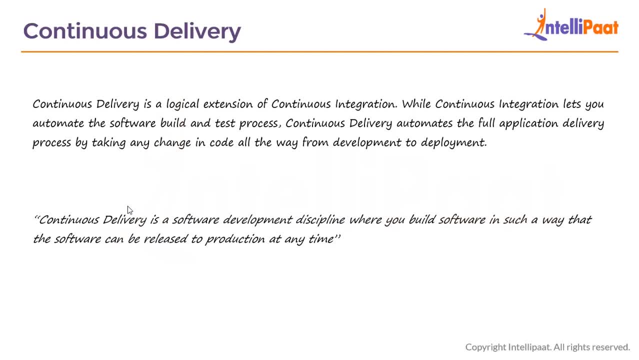 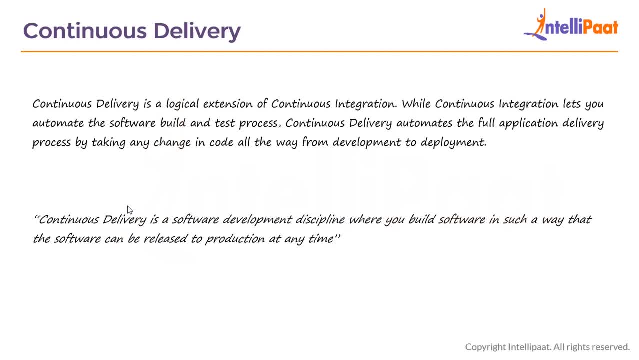 That is the code commit part To deployment, which includes deploying them to environments such as staging and production. It also ensures that you are able to release new changes to your customers quickly, in a reliable and a repeatable manner. So, according to Martin Fowler, who coined the term, continuous delivery. 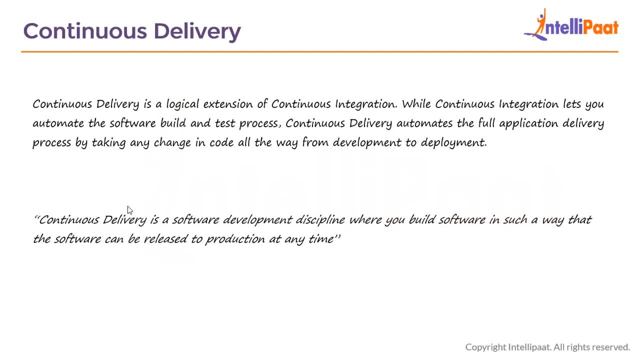 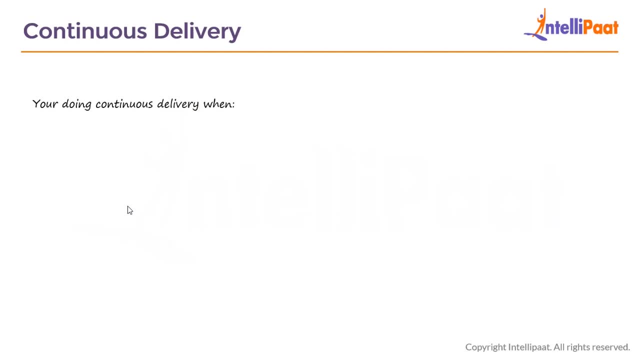 He says continuous delivery is a software development discipline where you build software in such a way that the software can be released to production at any time. So you are doing continuous delivery when you follow some of these steps. Now let us take a look at some of these steps. 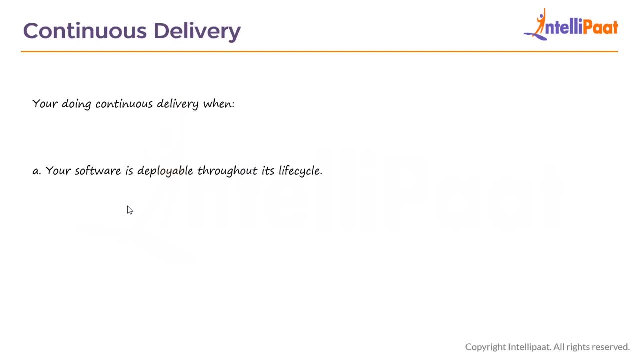 The first one is your software is deployable throughout its life cycle. Then your team prioritizes keeping your software deployable over working on new features. Anybody can get fast automated feedback on the production readiness of their systems anytime somebody makes a change to them. 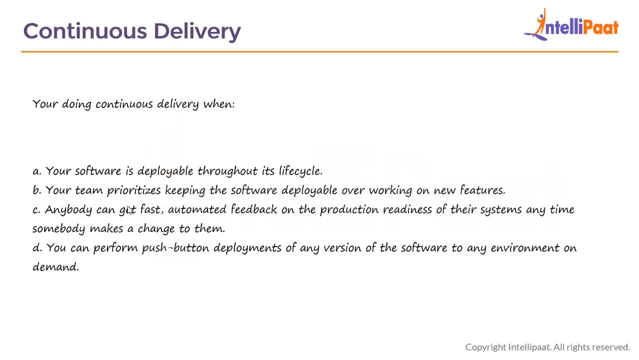 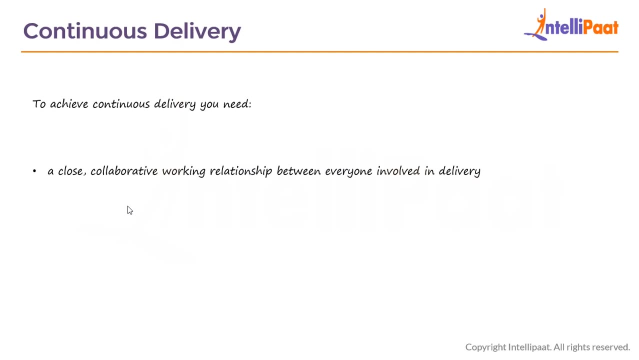 You can also perform push button deployments of any version of the software to any environment on demand. And then to achieve continuous delivery, you will need two of the following steps, which is a close, collaborative working relationship between everyone involved in delivery, So this often is referred to as a DevOps culture within an organization. 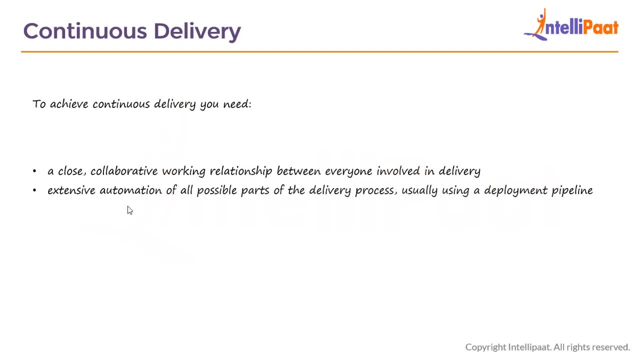 Then you need an extensive automation of all possible parts of The delivery process, usually using a pipeline, which is can also be called as a deployment pipeline. Incorporating continuous delivery practices will make your overall release process painless, reduce the time to market for new features and increase the overall quality of the software, thereby leading to greater customer satisfaction.